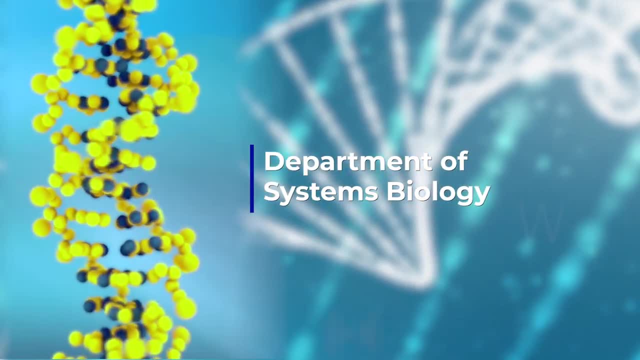 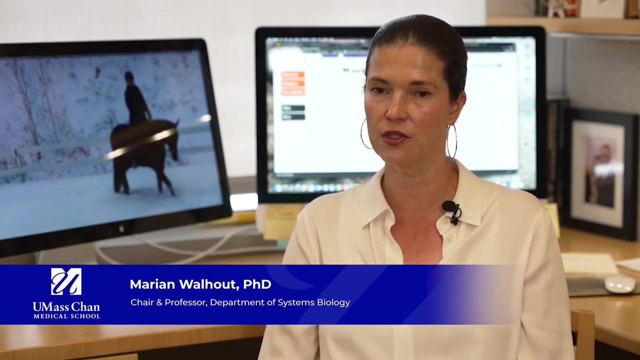 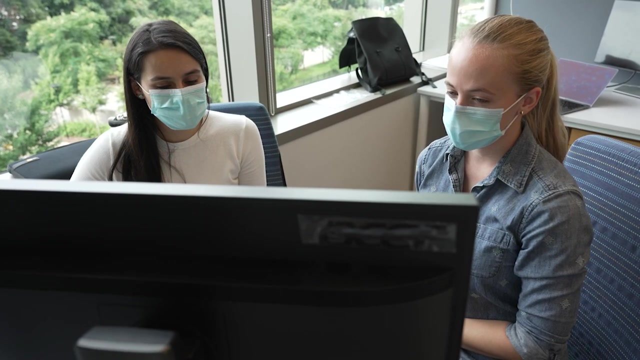 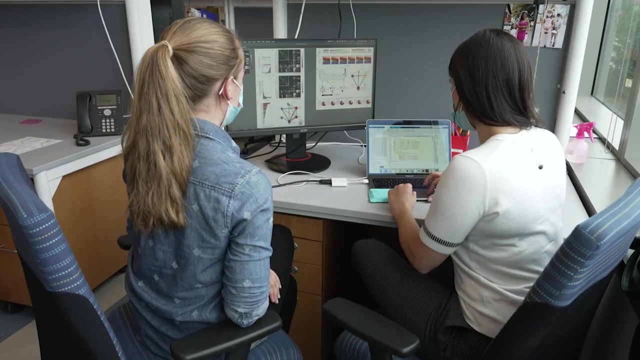 In systems biology. what we try to do is combine large data sets and many different, often quantitative, observations to gain insight into healthy biology as well as in disease. And for students, I think this is very exciting because it offers the opportunity not only to learn biological techniques, biological disciplines such as genetics and biochemistry, but to combine. 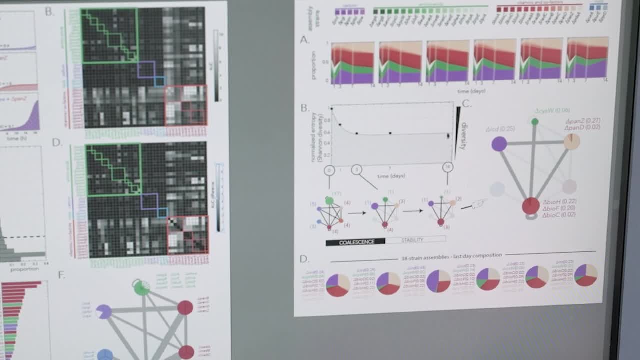 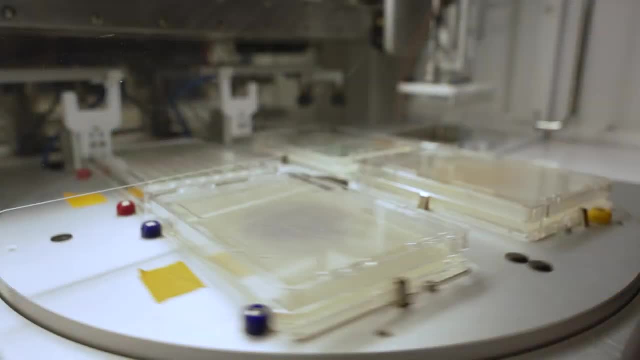 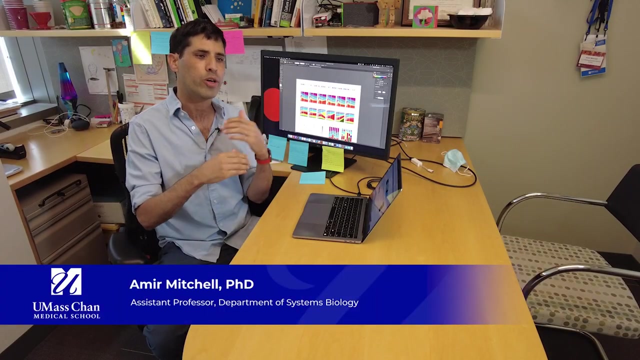 that with computational modeling, statistics, physics and so on, to gain both broad insights into biological processes and disease, as well as to go deep into different mechanisms and therapeutic interventions. We need to understand biology and the organizing principles behind biology, not just by focusing on a single gene or a single organism or a 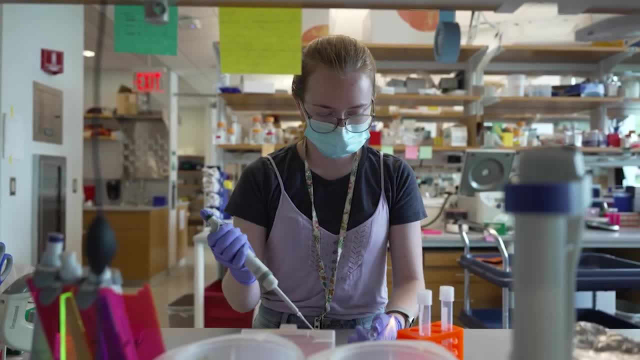 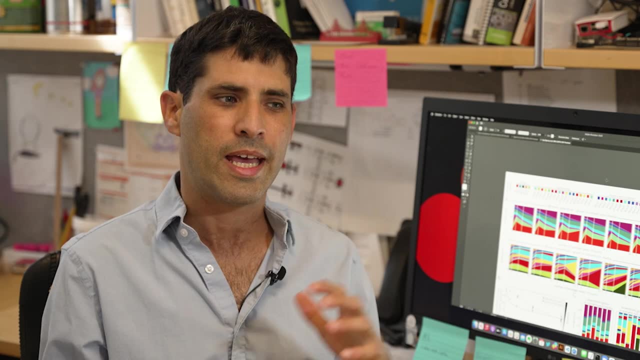 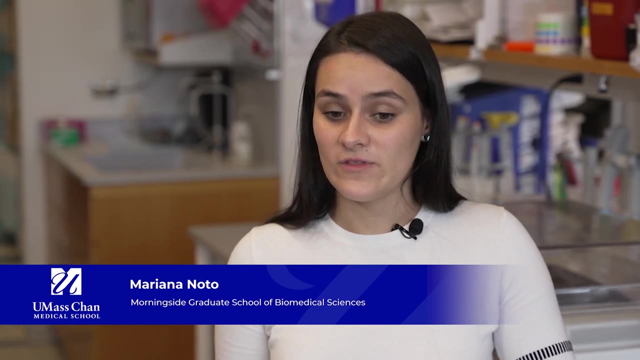 single model system. We're trying to understand the very basic foundations of biological systems or the principles in which they are all operating, and this department is really the perfect place to do that. I use genomic approaches to understand the metabolic interactions that happen in microbial 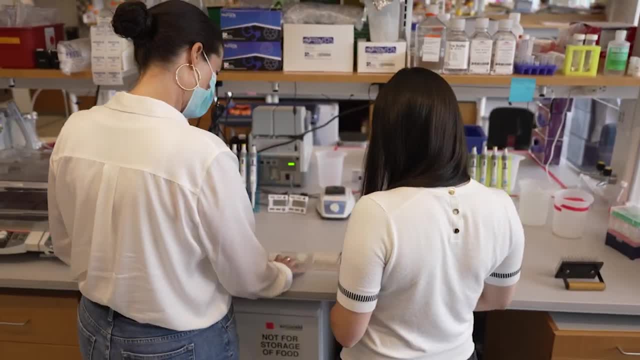 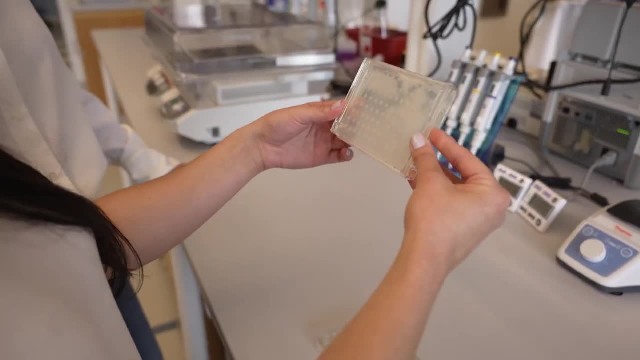 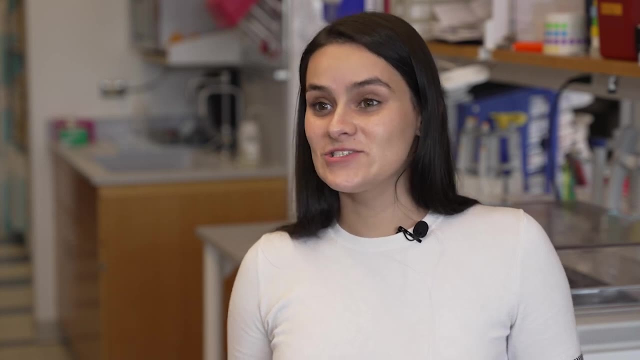 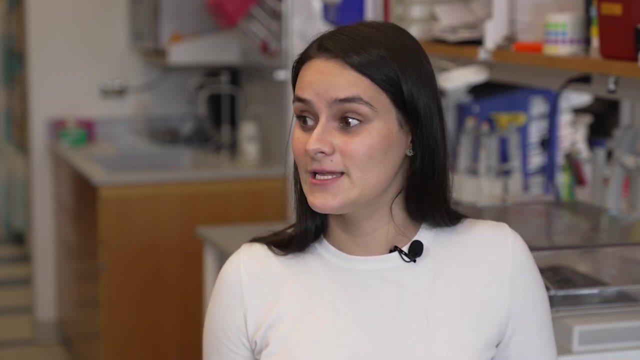 communities. My goal is to try to understand the design principles that underlie cross-feeding interactions in microbial communities And then to test these principles by assembling synthetic communities in the lab. The Systems Biology Department is truly a very collaborative and friendly environment. As you see, it's an open space where we can share and learn from everybody's work. 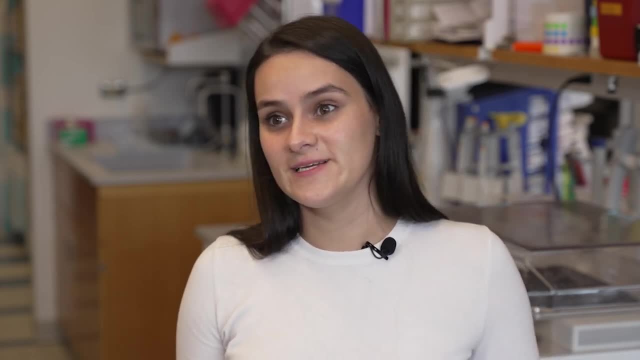 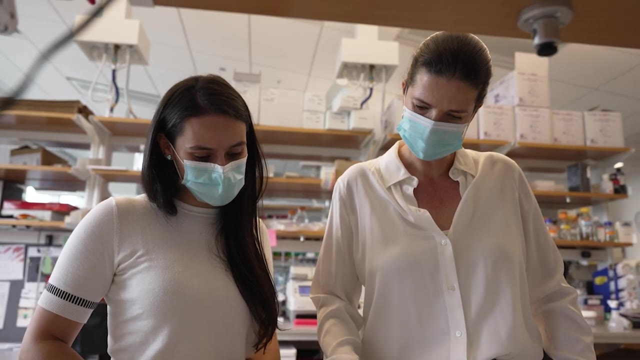 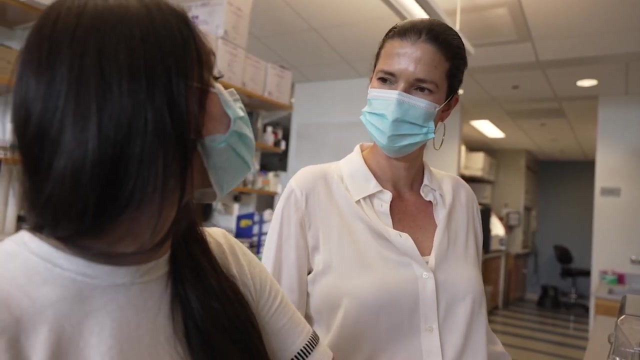 And also we are part of a very fun and supportive environment. We are exposed to a lot of different experimental strategies, And whenever we're trying to set up new things, we can always walk across the benches and ask for help, even from people that are not in our same lab. 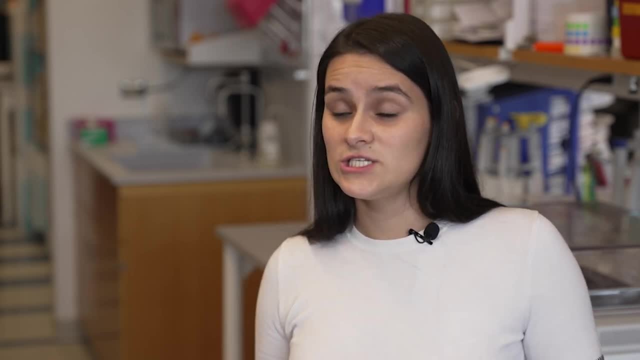 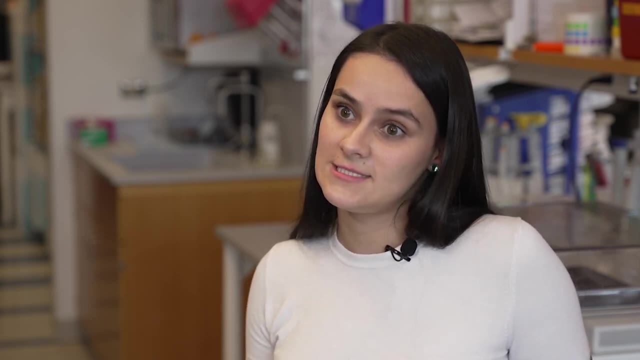 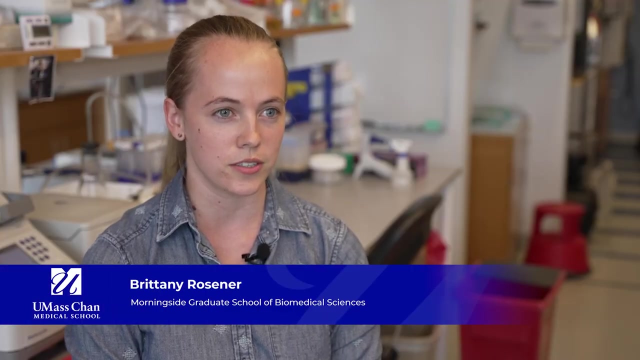 I have learned to set up high-throughput experiments, genetic screens, next sequencing protocols, and also I acquired the computational skills that allow me to perform data analysis. I study the complex interactions between bacteria, drugs and hosts. Specifically, I'm interested in the microbiome.